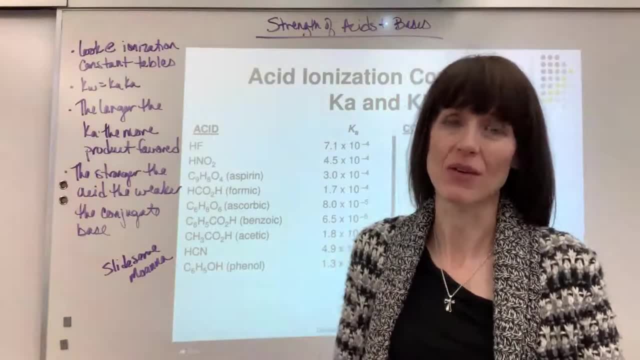 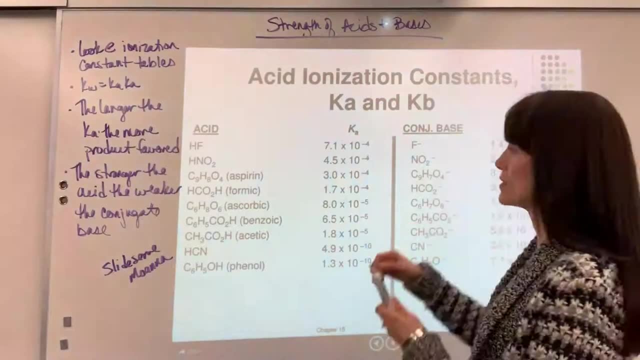 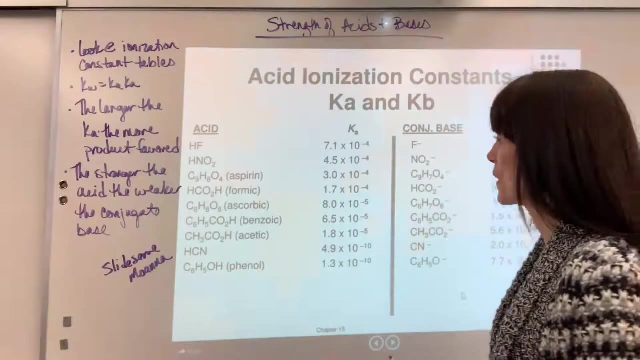 Hi, I want to compare the strength of acids and bases with you. Here's the key. You need to look at an acid ionization constant table. This one is just a little snippet of one and many things through SlideServe Moana. If you want to look this up, you can google that. So it is giving us. 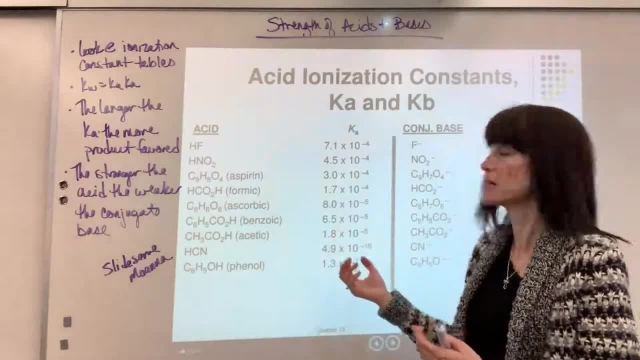 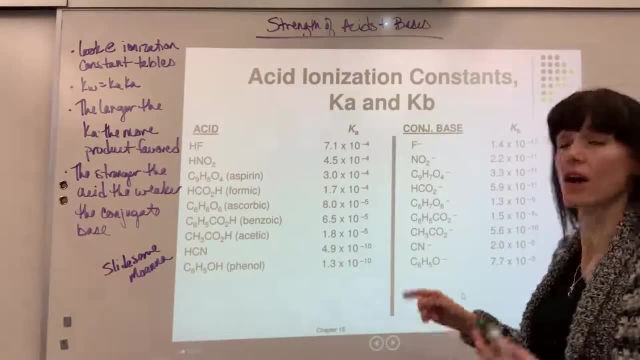 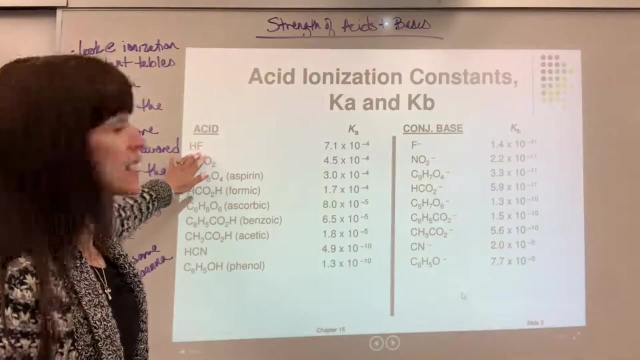 our Ka values. so the equilibrium constant, the ionization constant for our acid reactions. You'll notice hydrofluoric acid, nitrous acid, and then over here we have our conjugate bases. So if the acid remember going to donate a hydrogen, this acid HF loses a hydrogen and its conjugate base. 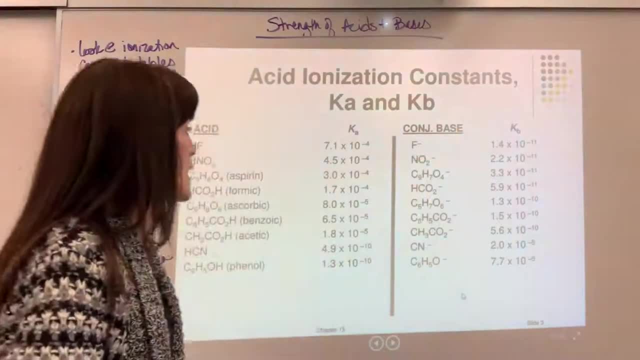 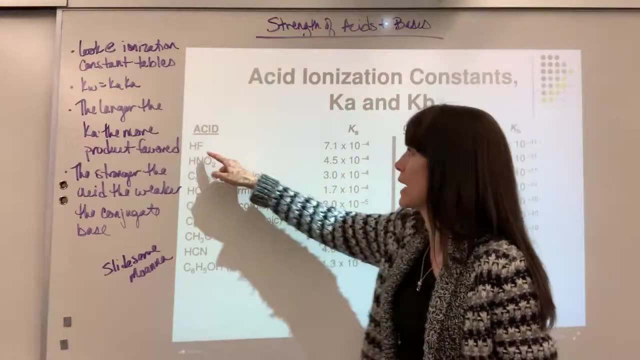 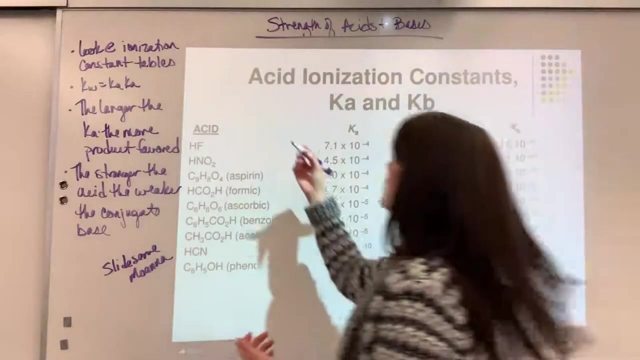 is going to be F minus one. It lost that hydrogen And you know, think about it. reverse: A base is going to accept a hydrogen. This is a base because it will accept a hydrogen to become HF. So this is looking at if that HF reaction was water, If we had this reaction is really what this is talking. 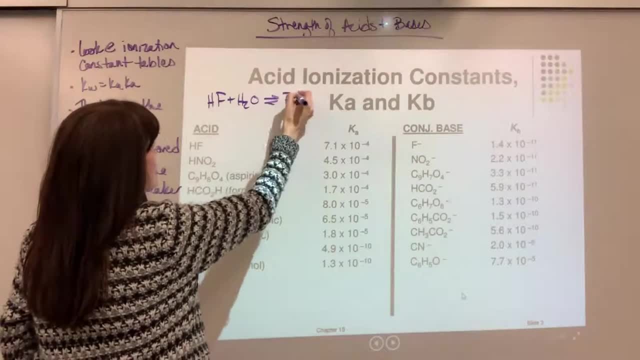 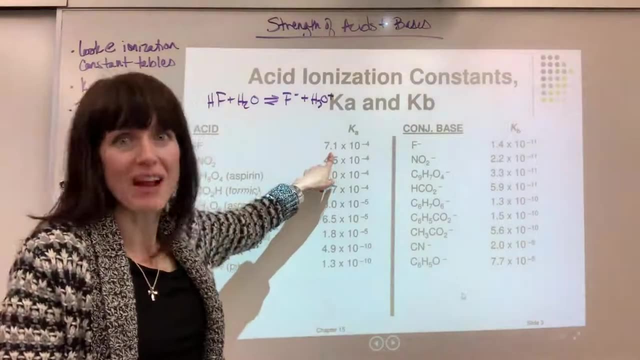 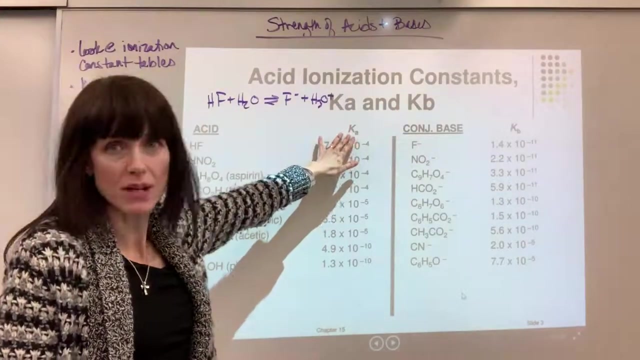 about Plus. water is an equilibrium with F minus plus H3O plus. This is the reaction for that number right there. This is the equilibrium expression You'd be. products divide by reactants equals that equilibrium constant. ionization constant- That's our specific word for acids. 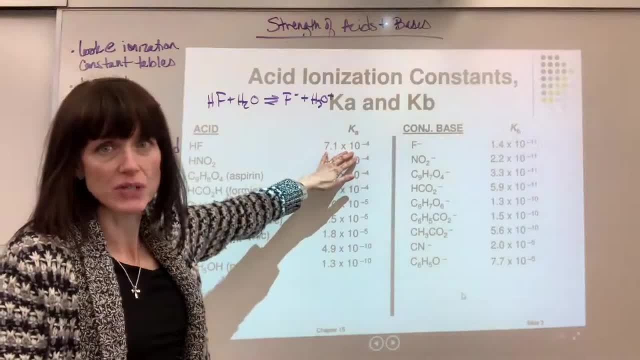 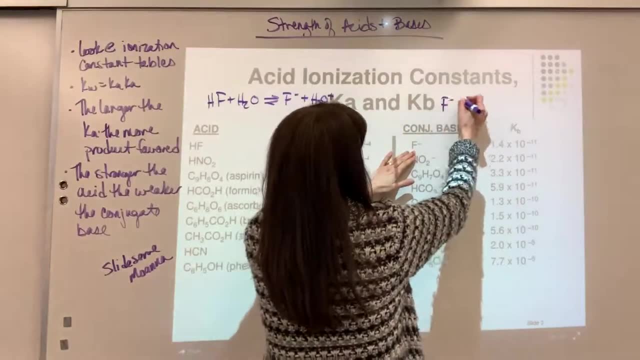 and bases, It is 7.5.. 1 times 10 to the minus 14.. That's how you interpret this. Now, this one over here. the reaction would be that fluoride ion plus water- Remember that's a base going to accept. 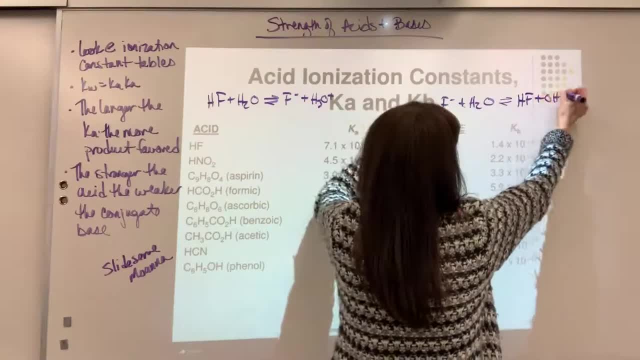 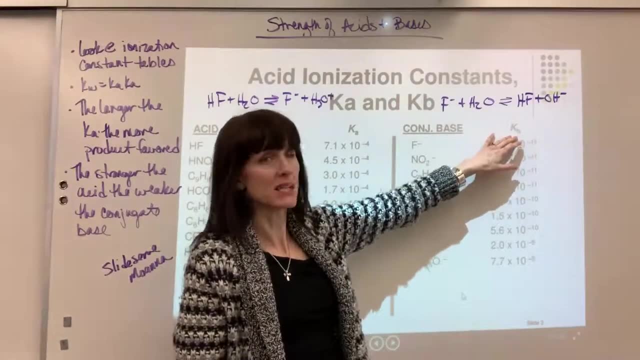 It's going to be equilibrium with the hydrofluoric acid plus the OH. Now this equilibrium- expression products over reactants- is going to give us a KB, the base ionization constant, of 1.4 times 10 to the minus 11.. So that's how you interpret one of these things. So if you have a base, you're going to accept a hydrogen. 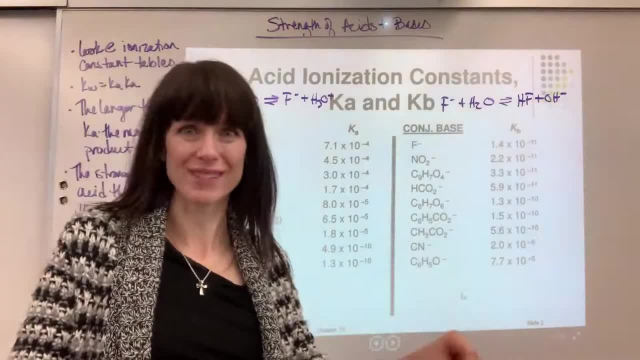 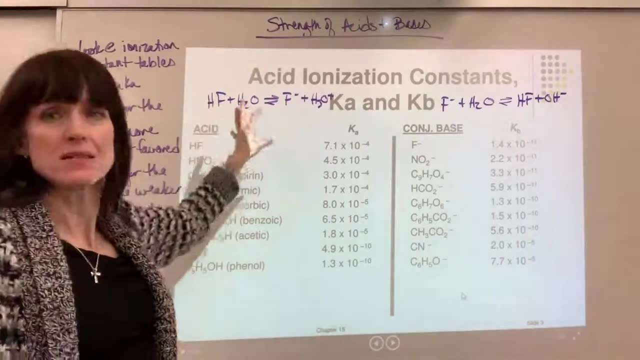 So if you have a base, you're going to accept a hydrogen, And this is the equation that I just explained today. Now, in this equation, you can write out the rest of that equation. This equation is pretty easy. You just know: acids donate that hydrogen, Bases accept that hydrogen. 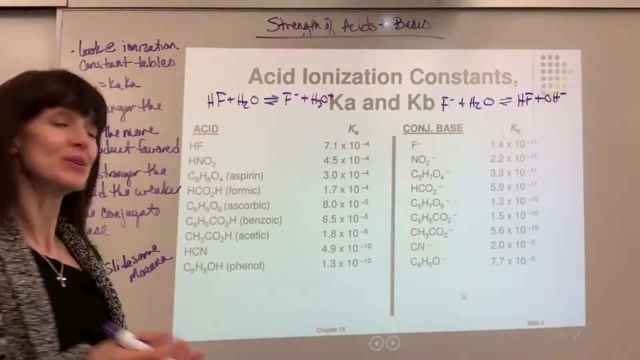 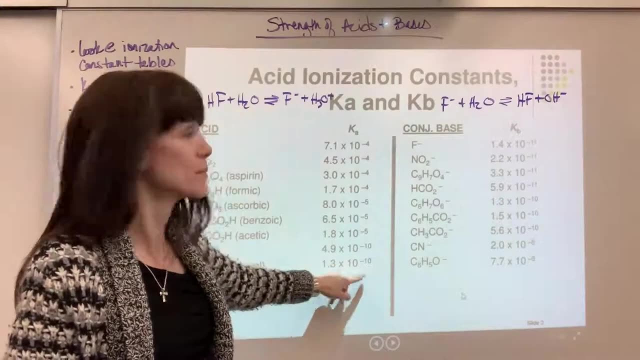 That's from our Bronsted-Lowry. Now notice the numbers on this Here, our KAs. as you go down, the numbers get smaller. Remember these are negative values. So negative 4 compared to negative 10.. 10 to the negative 10 squared. 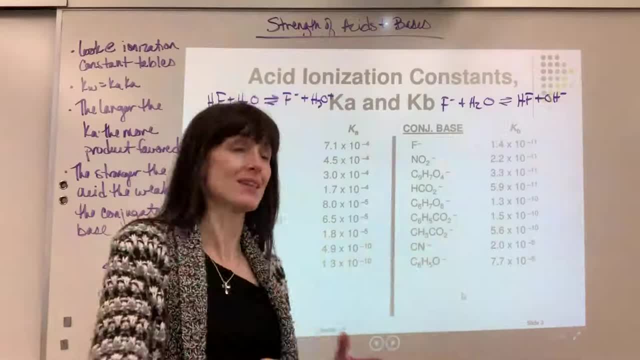 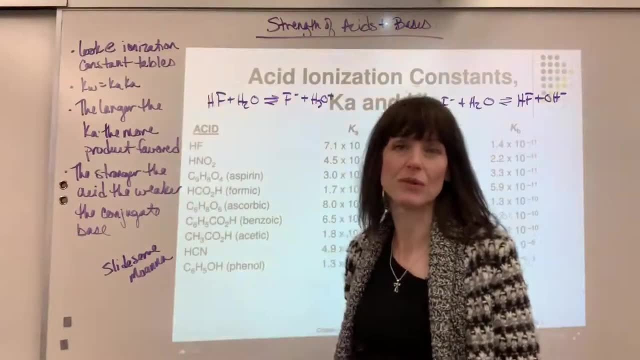 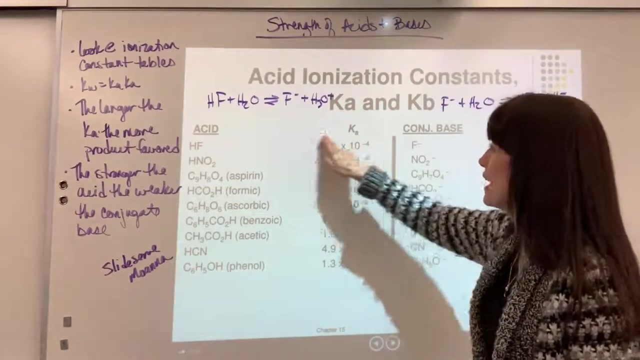 may be smaller. Over here on the base it's just opposite. We have the negative 11 going down to the negative 5.. Why is that? It comes back to this: Kw equals Ka times Kb. So when you multiply- pretty neat- the acid ionization constant times, the base ionization constant, guess what They? 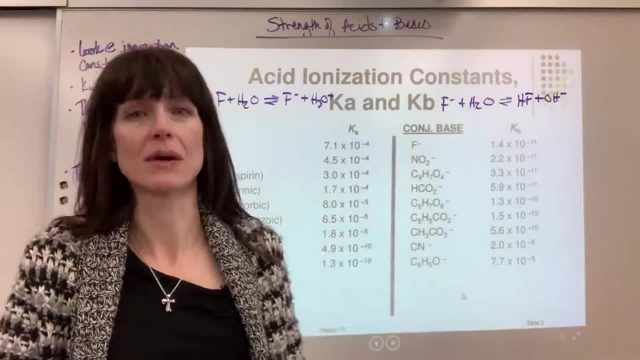 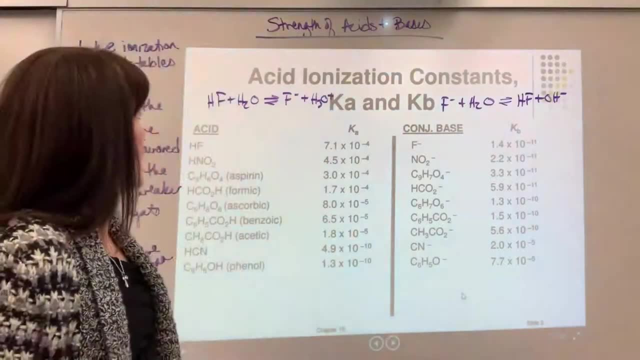 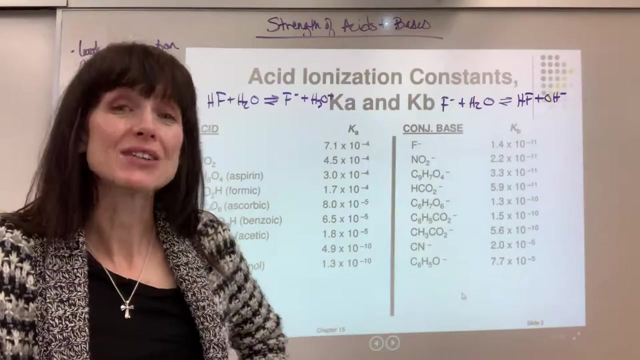 always equal Kw, which is 1 times 10 to the minus 14.. Watch that video in the acid-base equilibrium playlist if you have questions. It just says acid-base ionization constants. Okay, so the relationship: they're indirectly related, As one is larger, the other one is smaller. 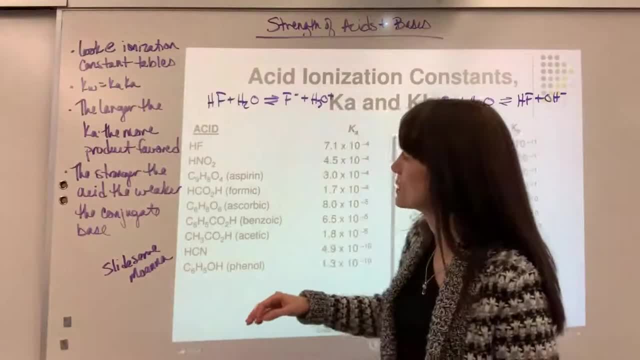 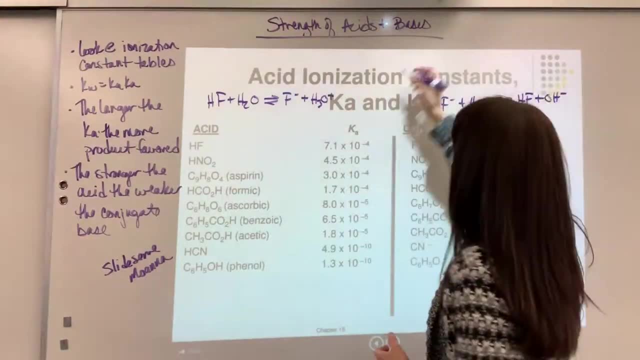 Now another big takeaway. I want you to look, as a reminder, right here: The larger the K value, the more product favored it is. You know this. When I do products over reactants, K greater than 1 is product favored, K less than 1. 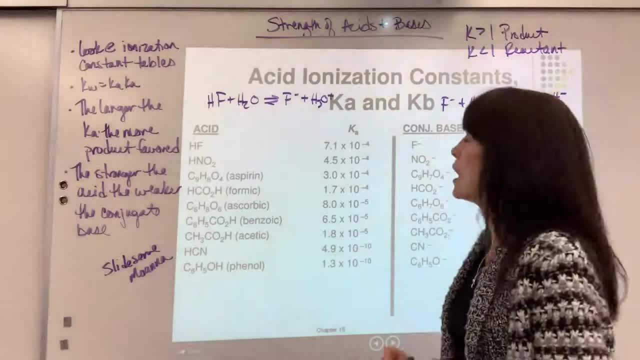 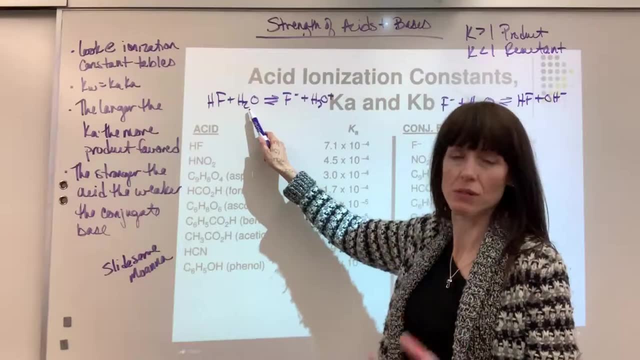 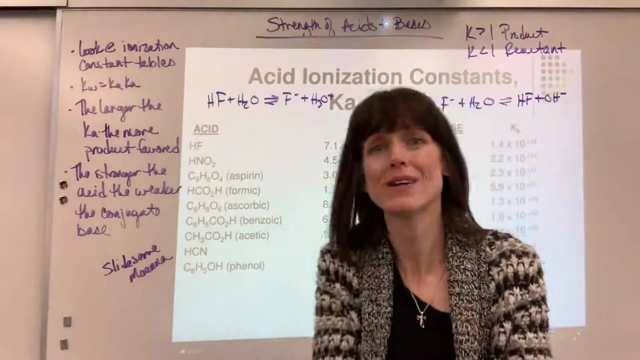 is reactant favored. So the bigger the number, the more products, the more that this species will react with water. Okay, so the bigger the number, the more it ionizes, the more it reacts. You recall all the weak acids and bases. they don't 100% react with water, Maybe only 5% will. 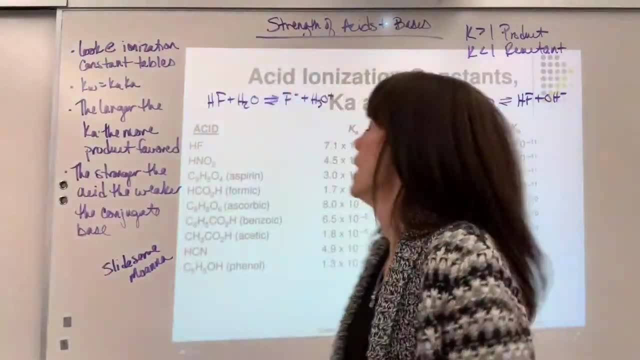 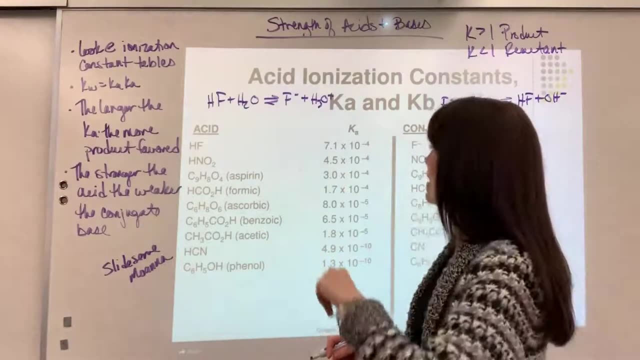 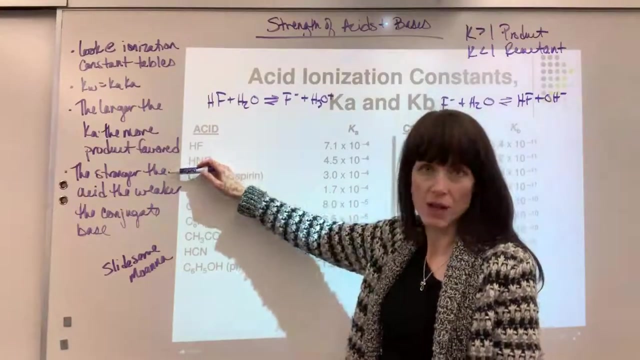 react. Strong acids, strong bases, 100% react. The 100% break apart, dissociate, ionize. Well, never mind on that. So, putting this all together, here are your big takeaways: The stronger the acid, the weaker the conjugate base, that indirect relationship. So the bigger the numbers. 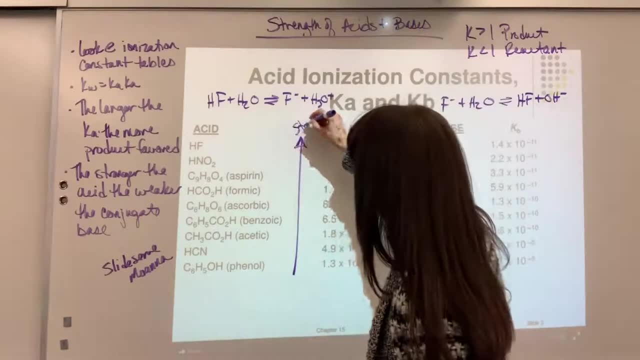 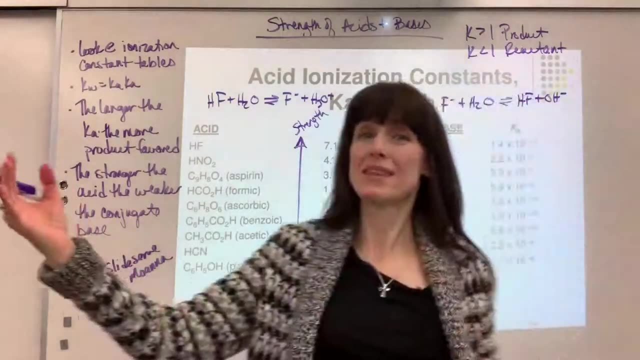 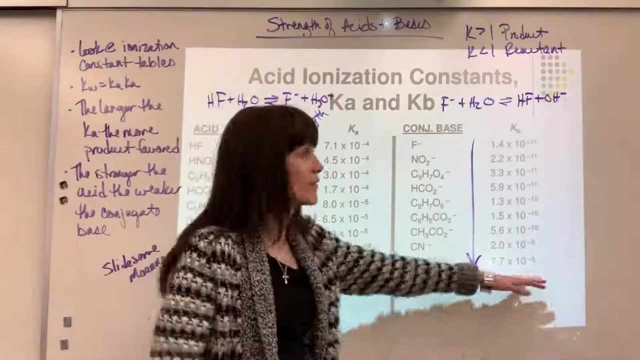 notice what I can do. right here We have an increasing strength for the acids as you go up this table, because our largest numbers are 10.. right here, So just opposite. the inverse relationship is: increasing strength is as you go down for the bases, because you have the biggest numbers at the bottom of the table. So this would 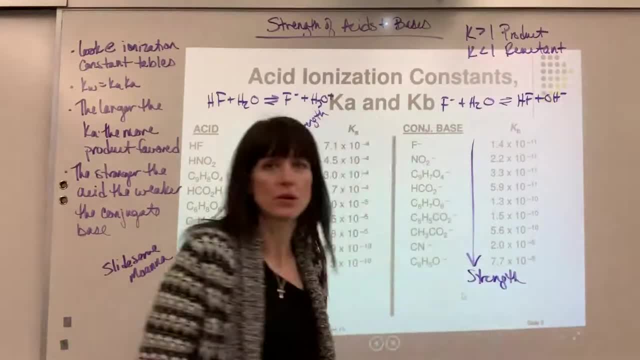 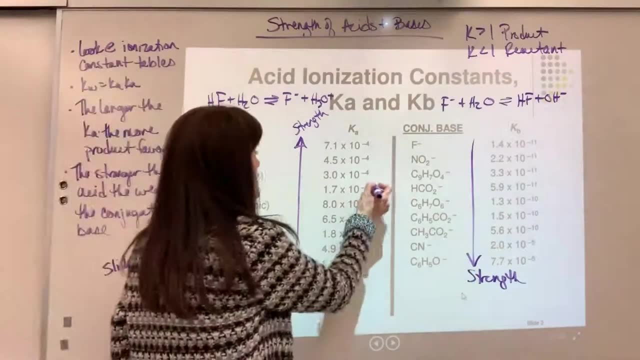 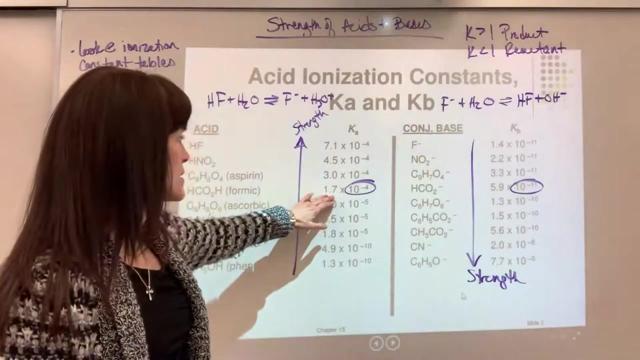 be your increasing strength as you go down, as you go down. So when I'm comparing my acid with my conjugate base, you're looking really at the exponents right there. So if we look at this formic acid, the acid is 1.7 times 10 to the minus 4 ionization constant, whereas the formate ion 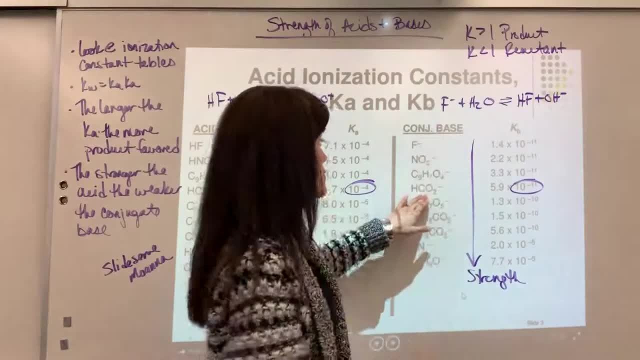 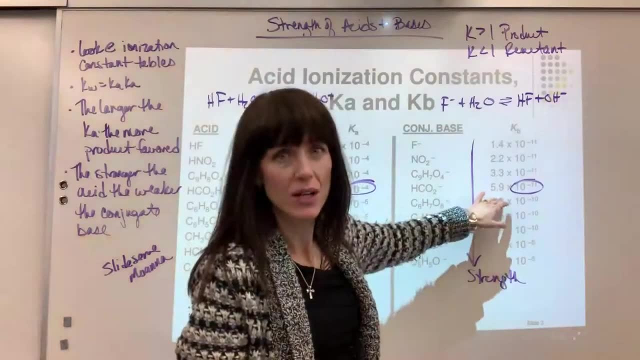 that would be that base reacting with water to produce the formic acid and the hydroxide. Okay, that base is 5.9 times 10 to the minus 11.. Well, the acid is much stronger than this base, So I. 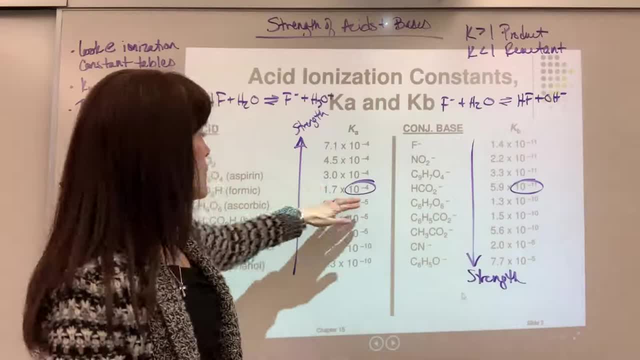 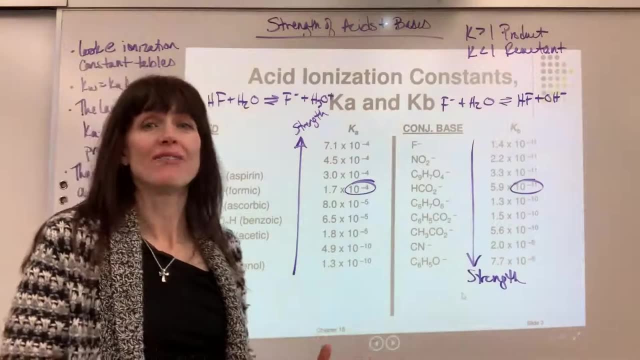 would predict that here, right here, this is going to be the base. So I would predict that here, this is going to be the base. So I would predict that here, right here, this is going to be the more product favored than this one would be this reaction over here. Okay now, if I can take just a, 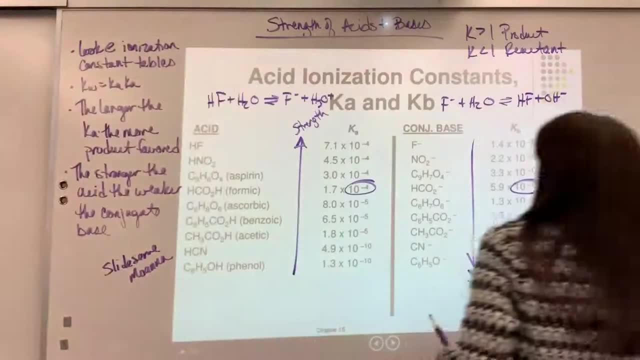 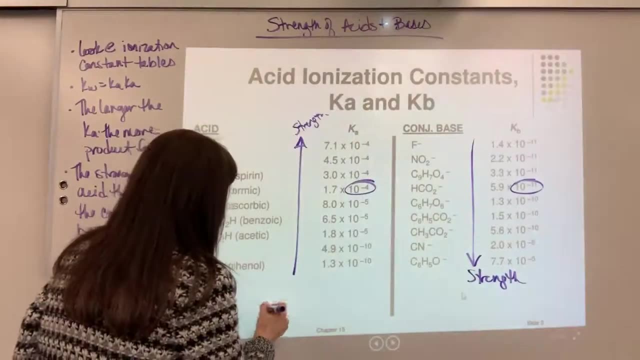 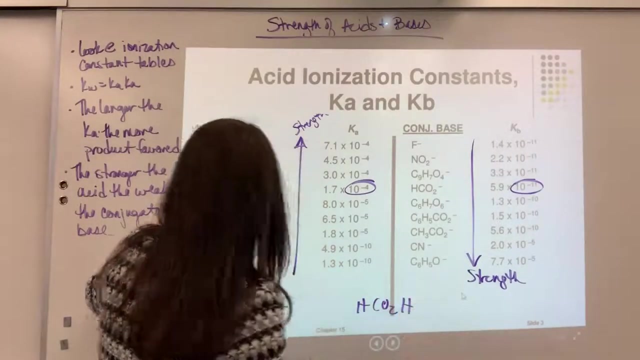 couple of these. let's take three, and we're going to compare them. Let me erase all this. Okay, let's take our HF, and then we'll go ahead and do our formic acid, CO2H, and let's do one more. Let's do this hydrocyanic acid. 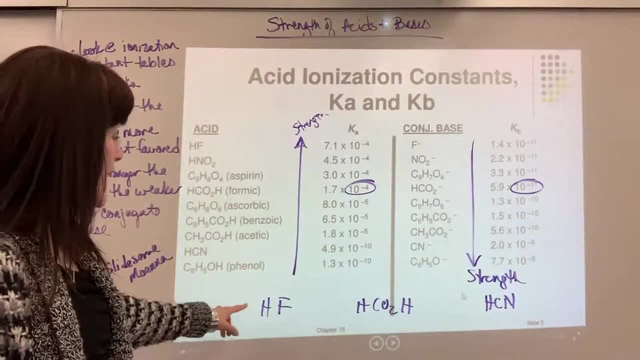 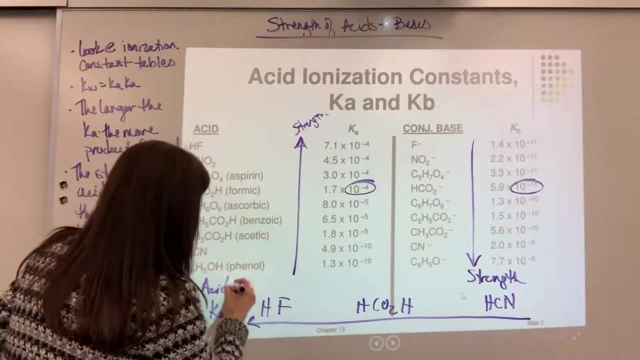 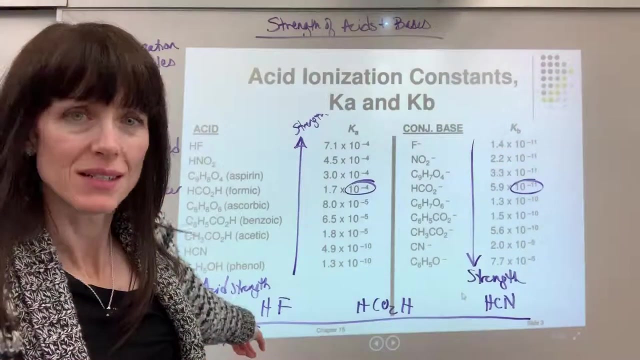 Okay, we know that the acid strength is going to increase this way for my KA acid strength. Okay, now I want you to think for just a second. why is that? Why did I draw the arrow that HF is the strongest Of all those acids? why is HF the strongest? It's because it has 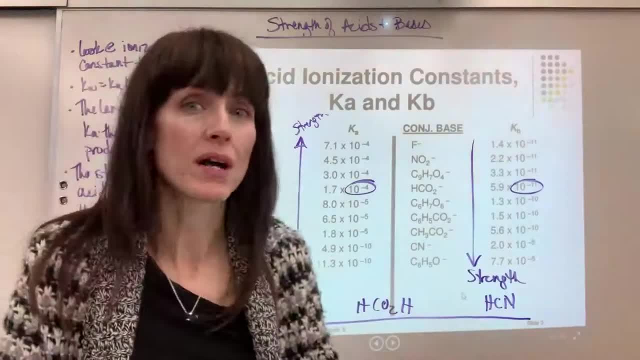 the largest KA value. It's going to break apart the most It's going to ionize the most. Because it ionizes the most it's going to break apart, the most It's going to ionize, the most It's going to. 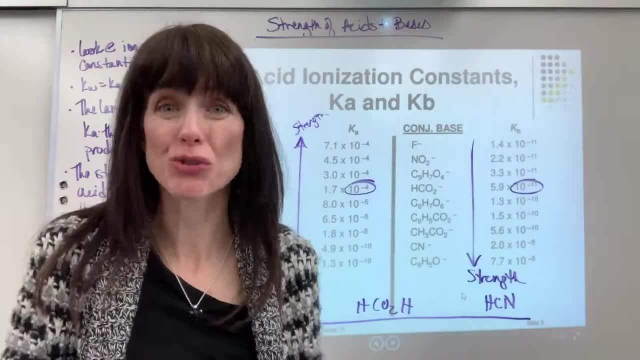 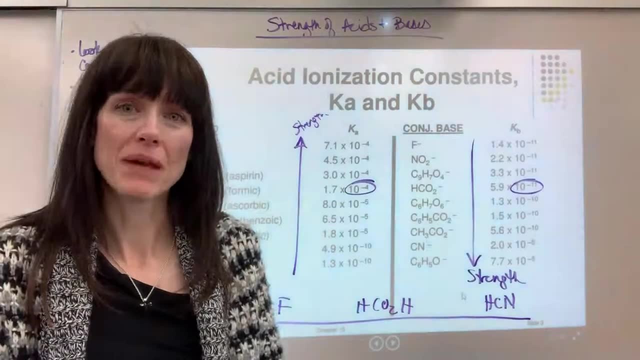 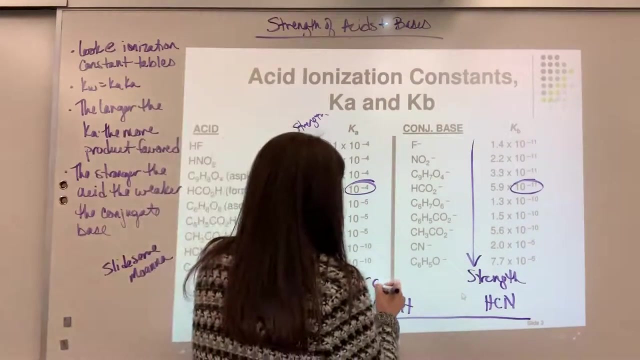 be the most ions available to react. So it's the strongest. Okay, so this would be considered the strongest. Now, just the opposite will be true for those conjugate bases. So let's take our. I'll put it up here. I have my F minus one, and then our formic ion, and let's do our. 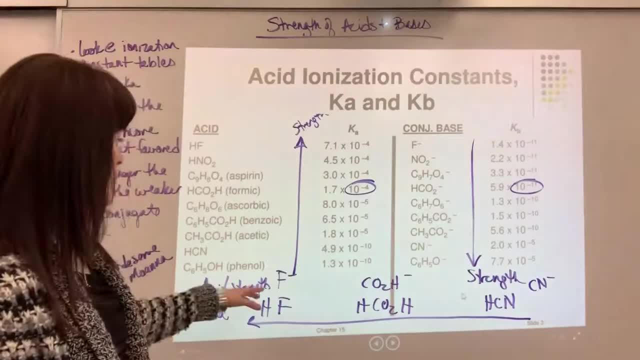 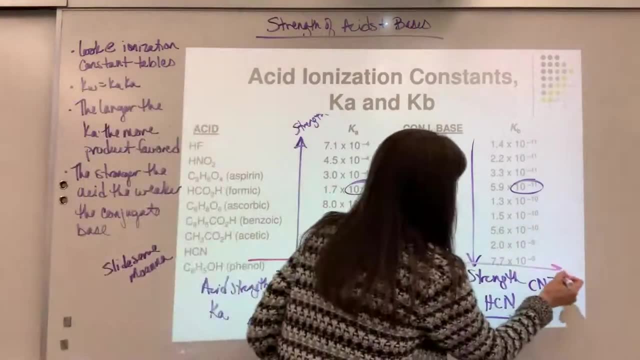 cyanide ion. So strength on this. if I'm looking at bases, let me do a different color for you. The strength of the base is going to be the strength of the ion. So if I'm looking at the bases, it's going to go this way And the cyanide ion is going to be the strongest base. 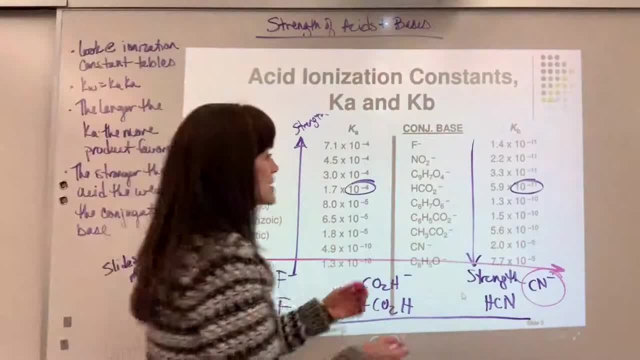 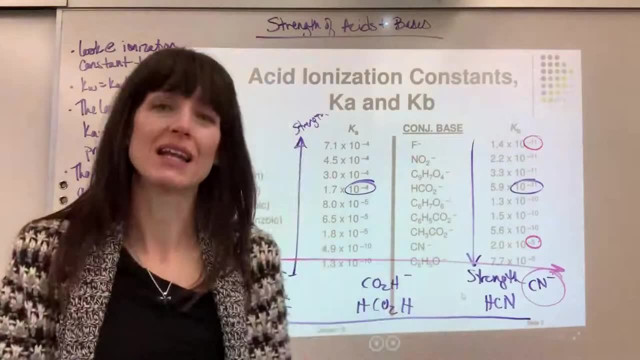 Why? How would you justify that? It's the fact that cyanide, wow, is 10 to the minus five compared to a 10 to the minus 11.. That is going to ionize more, is going to react more with the. 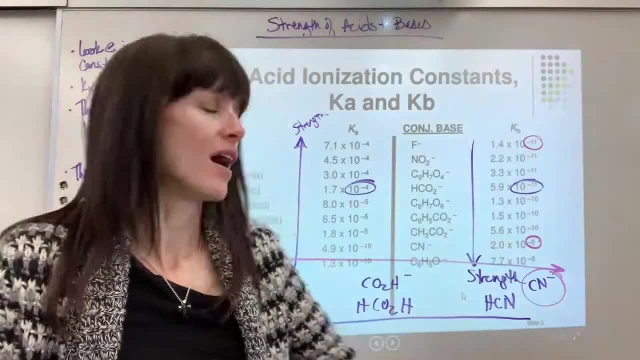 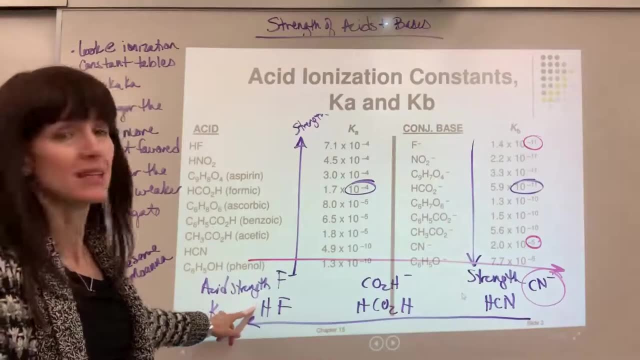 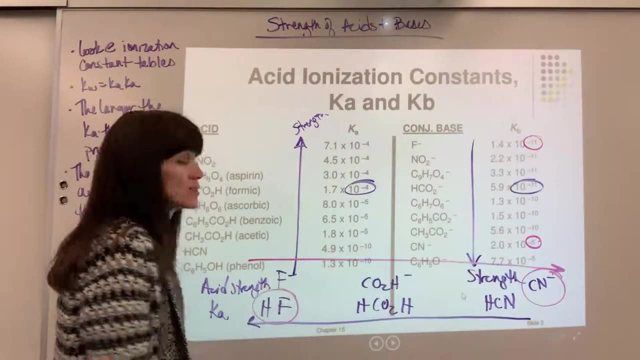 water, more ions available to do some chemistry, So this would be the strongest conjugate base, Whereas the HF is the strongest acid. Okay, so strongest base in this over here would be your strongest acid. Let me circle that one right there. So just looking at your numbers, So big. 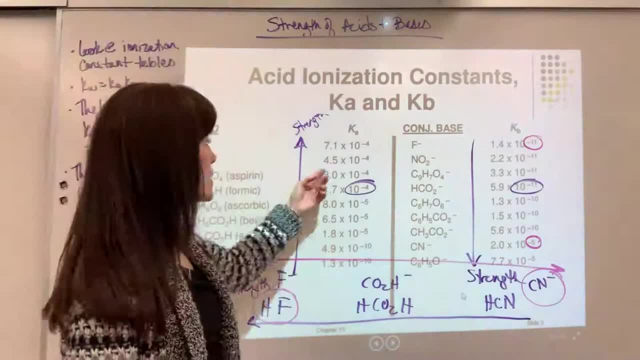 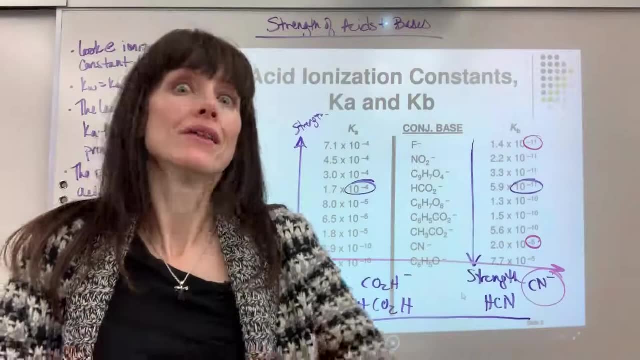 takeaway: when you're comparing acids, the larger the number, the stronger the acid. When you're comparing bases, the larger that KB, the ionization constant, the stronger it is. There you have it. It all depends on that ionization constant. 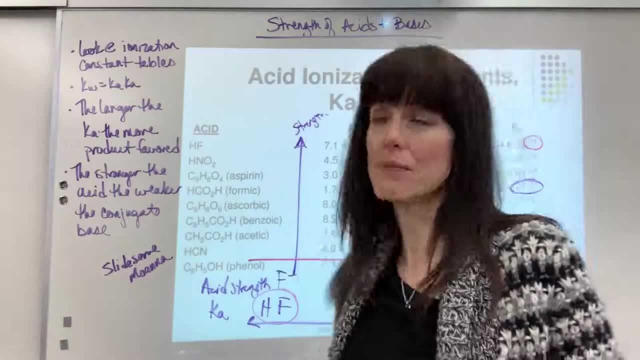 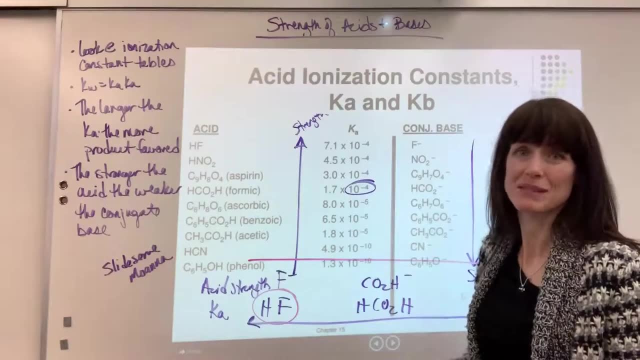 How much of it ionizes, reacts with the water. Okay, nice Hope that you are comfortable interpreting this. Bigger the number, the stronger the acid or the base. Okay, thanks, Have a nice day. 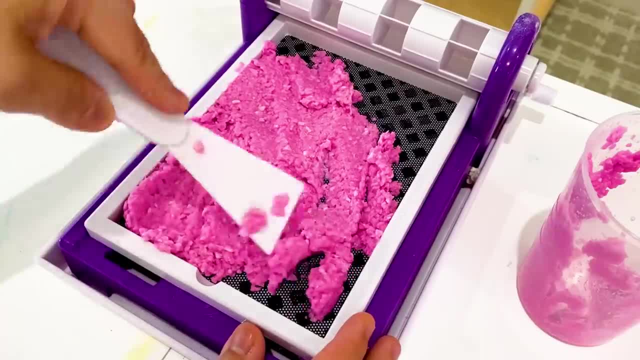 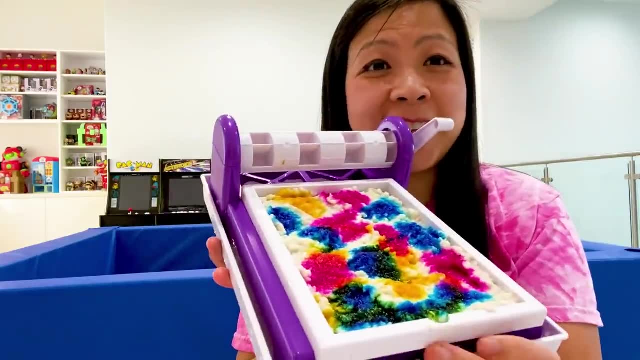 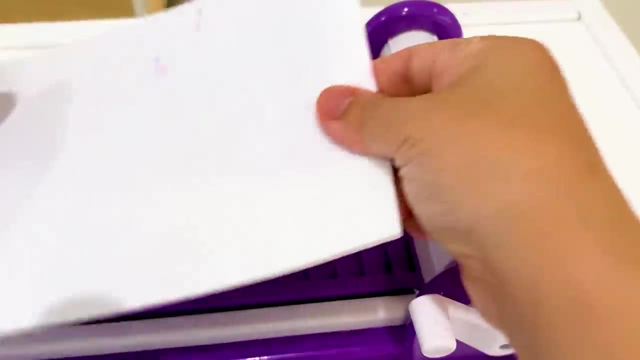 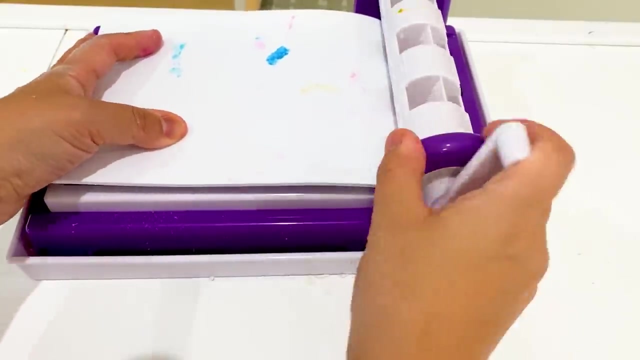 Next step is to pour the hope here and just spread them. Next, I'm just going to add some drops of colors. Look, Okay, that is so beautiful. Okay, next the mesh paper, this other thing, then the foam. Next, using all my strength, let's roll it. Who am I kidding? What strength.